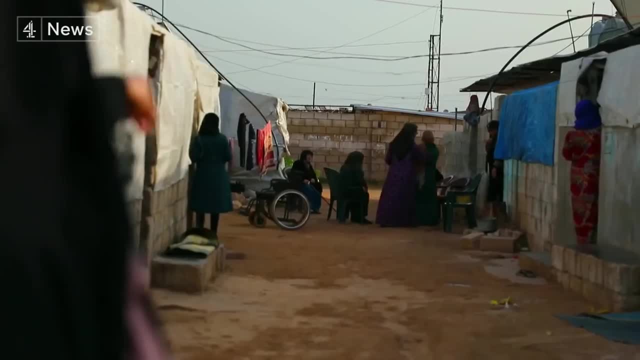 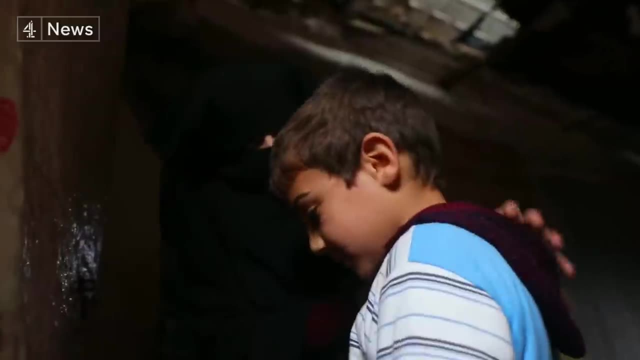 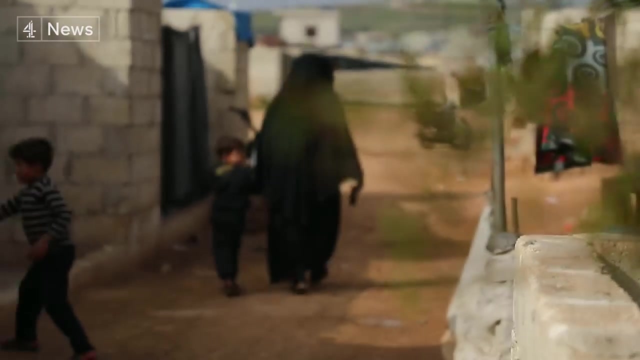 A hundred women live here with their children. The conflict has taken the lives of many of Syria's men, leaving the women to fend for themselves. But the death of a husband is not the only loss. A woman alone is often ostracized, left without any support. 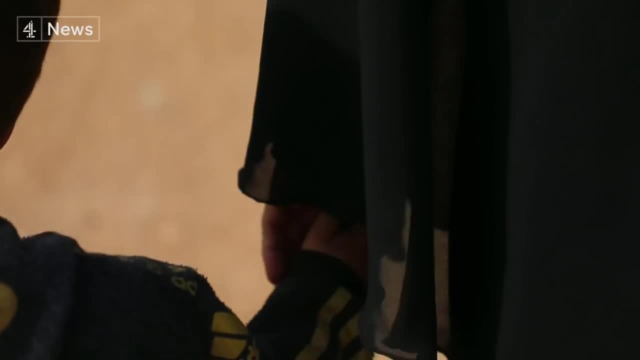 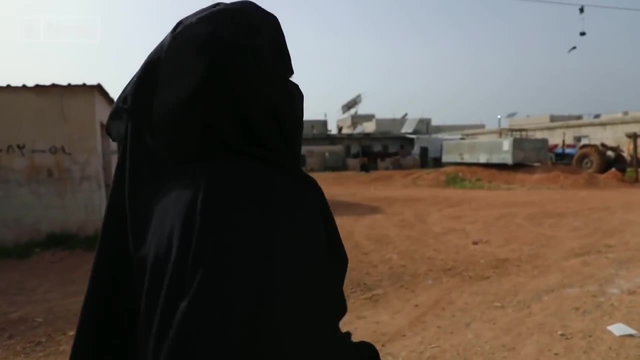 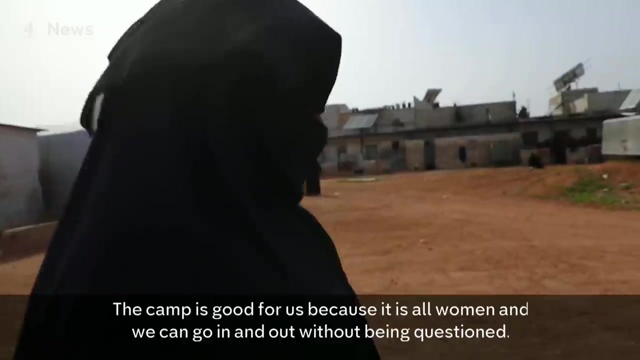 Umm Mohammed's husband was attacked, robbed and killed in Damascus. She came to this shelter with her divorced daughter and grandson. She had no money, no security, no choice. It is appropriate for us women to go out together. There is no one to tell you where you are going and where you are coming from. 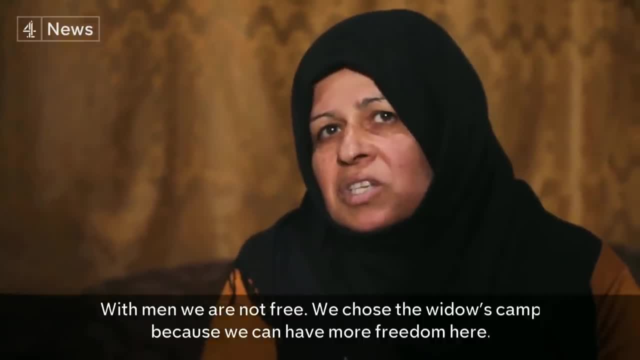 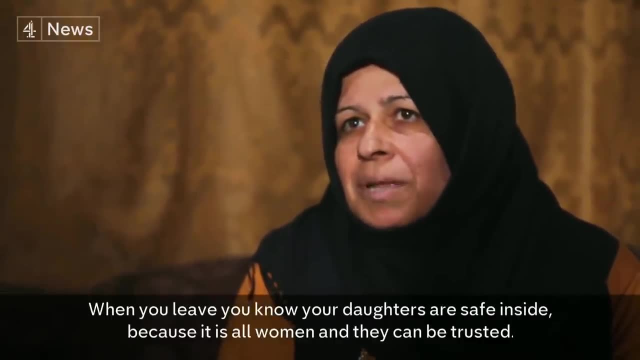 Because if there are men there, you do not want to take your freedom. Why did we take the camp of Arameel? Because you take more freedom in the house, You go out and you secure your daughters. All women are secure in it. 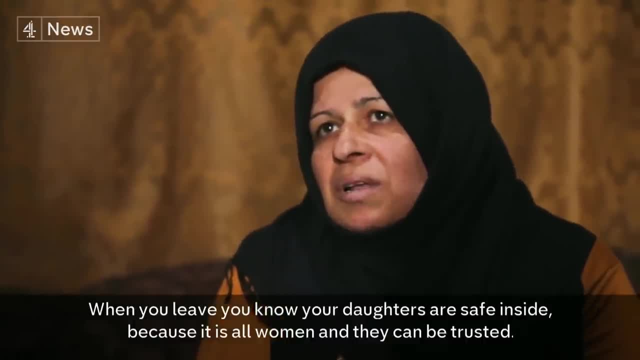 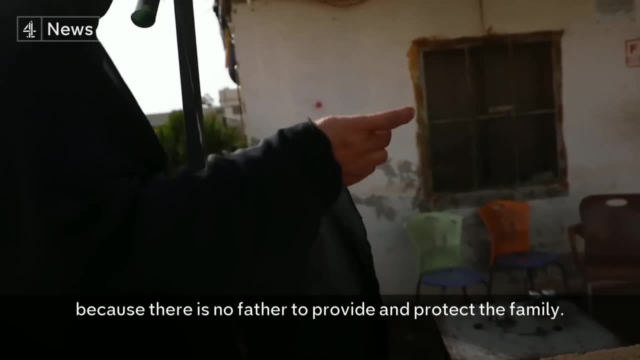 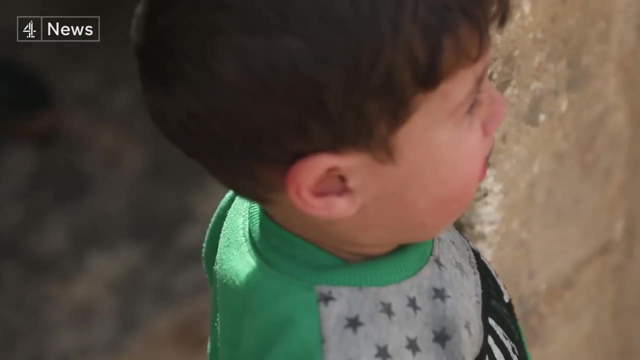 If you enter, you are secure. Thank God, all women are very strong Because there is no father who suffers and suffers. No one enters, No one looks at you. But the freedom she speaks of is limited. The gate of the widow's village is guarded. 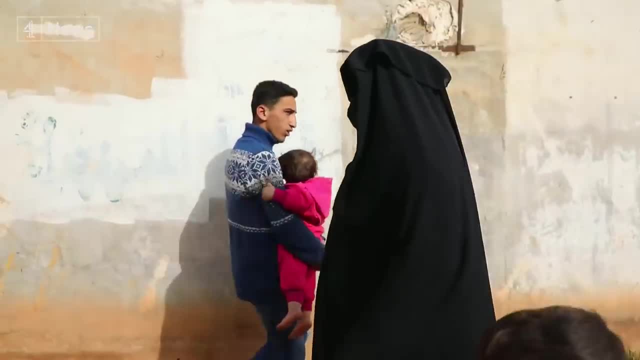 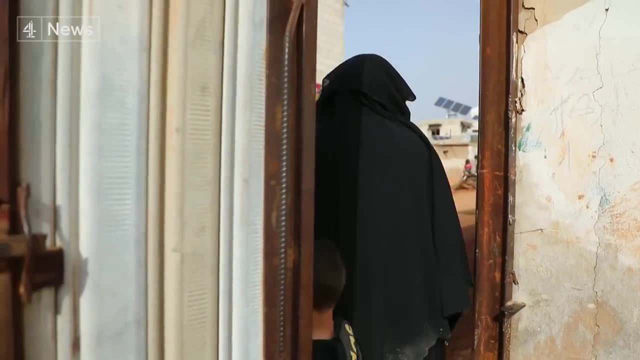 Inside the laws are those of HTS Hayat Tahrir al-Sham, the Islamic jihadi group linked to al-Qaeda in the past and now in control of Idlib. The conservative Islam they preach makes independence for these women difficult. 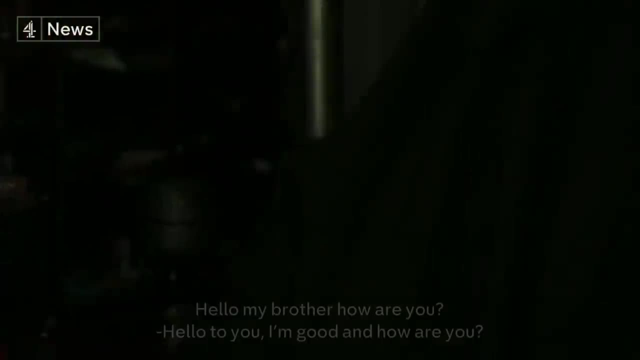 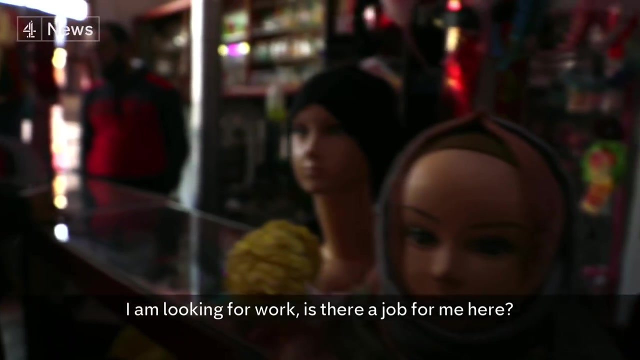 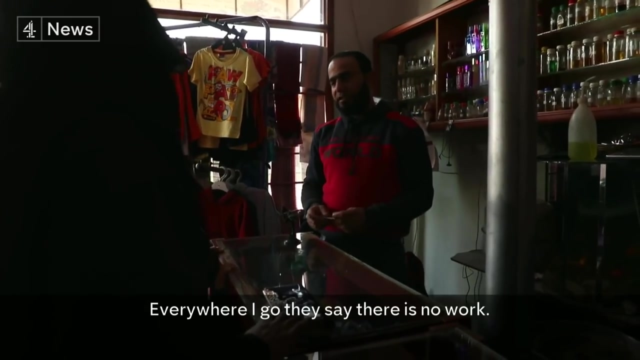 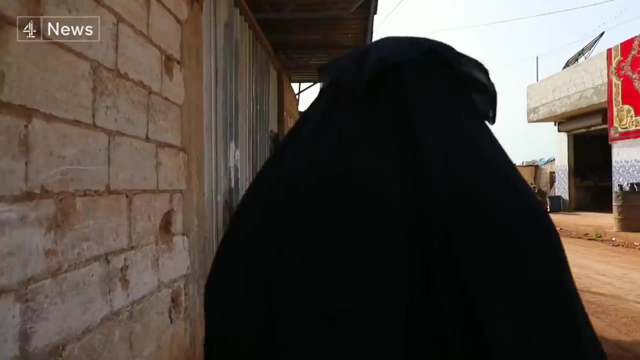 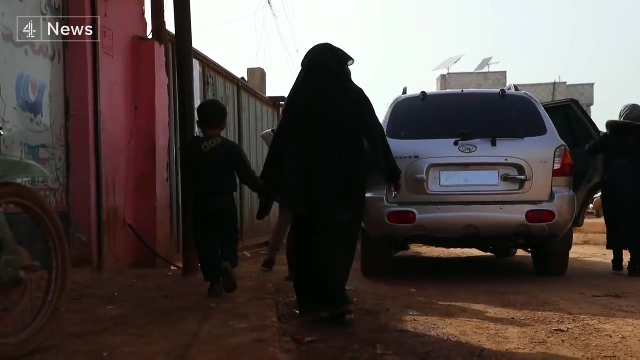 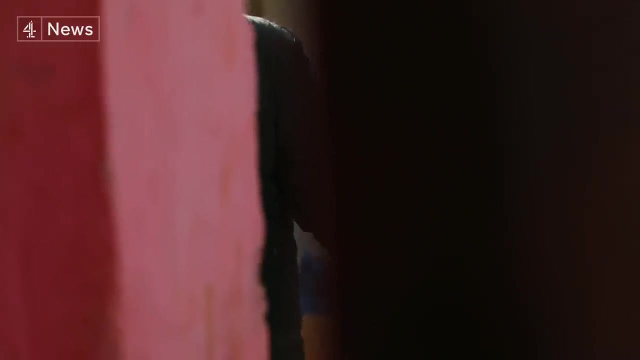 成 Seiqqa. So Um Muhammad is yet to find the work she needs to support her family financially for being a woman alone, one beyond money, and it is a price passed on to generations of women and girls. Amma Hamid says she has had to marry her daughters off young, a decision she bitterly regrets. 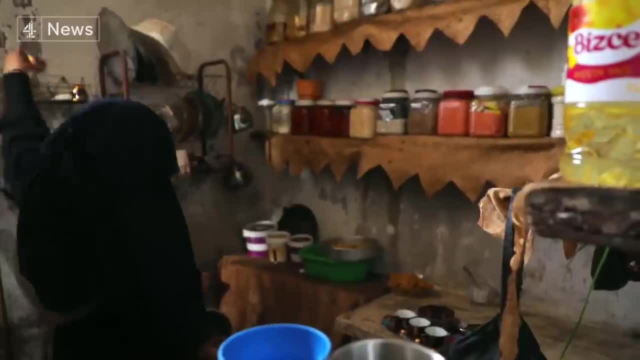 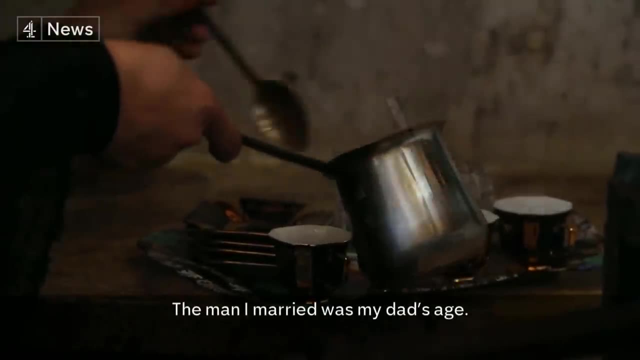 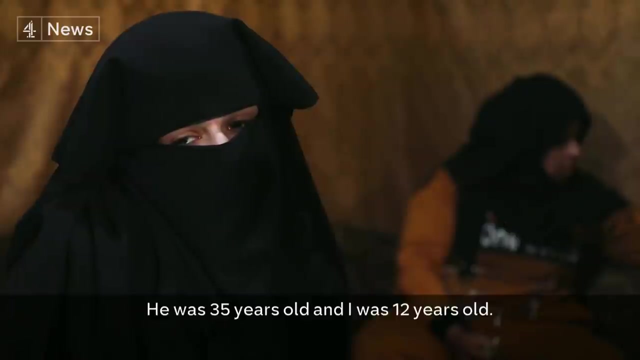 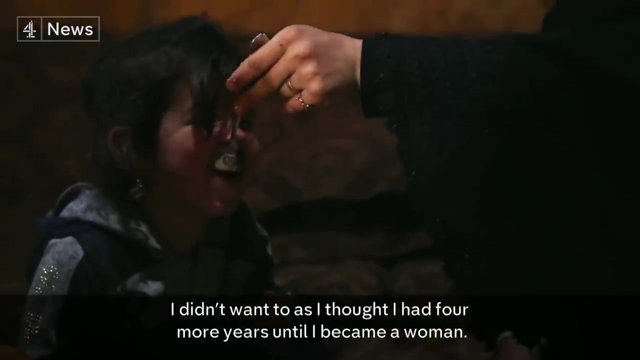 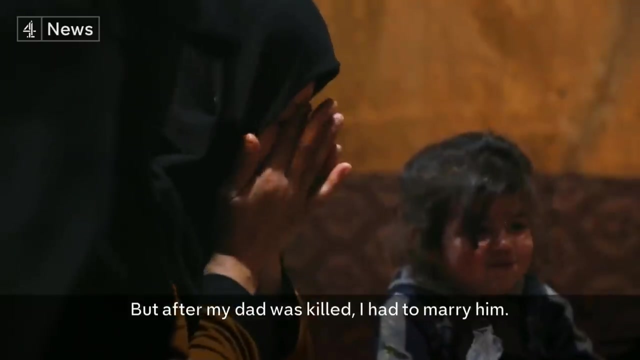 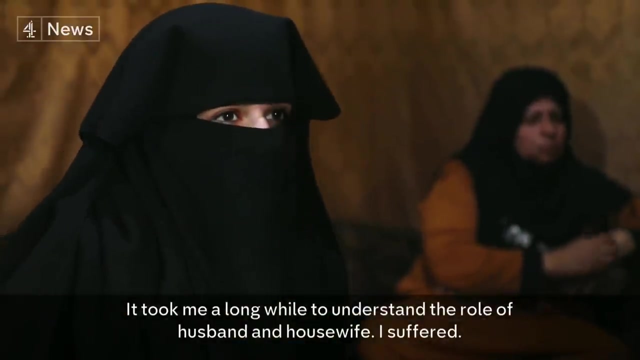 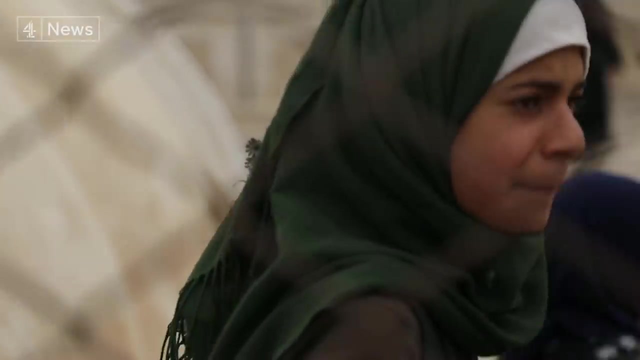 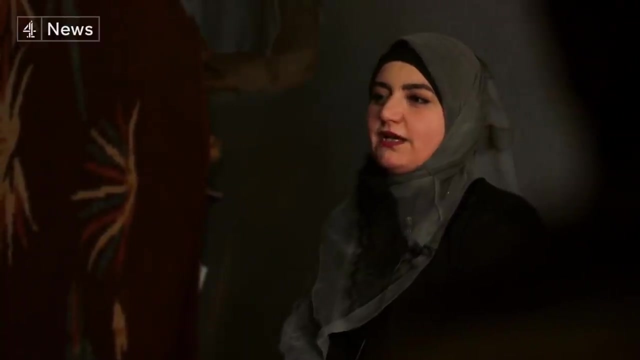 Amma Hamid's daughter, Ines, was just a child when she was forced to marry. There are attempts to break this cycle, to challenge the tradition of girls being forced to marry as children. Maisa's passion for her work driven by the trauma of her past. 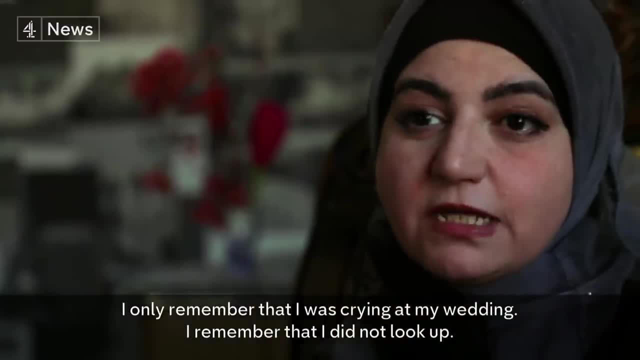 Amma Hamid says she was forced to marry her daughters off young, a decision she bitterly regrets. Amma Hamid's daughter, Ines was just a child when she was forced to marry. Amma Hamid's daughter Ines was just a child when she was forced to marry. 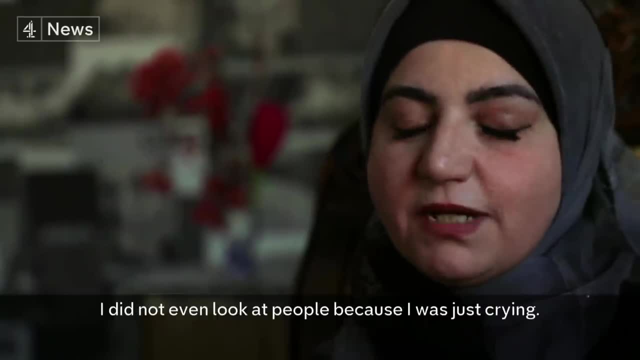 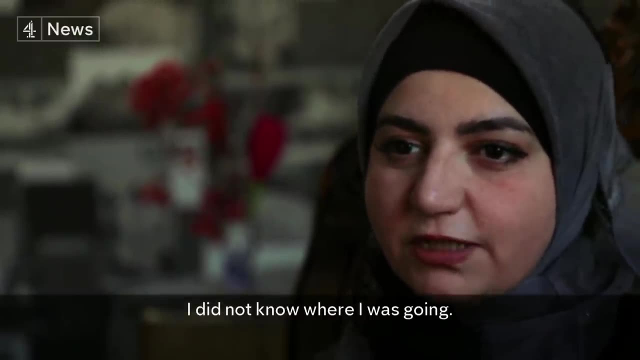 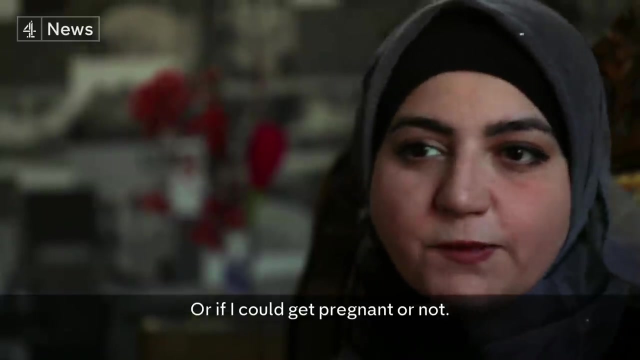 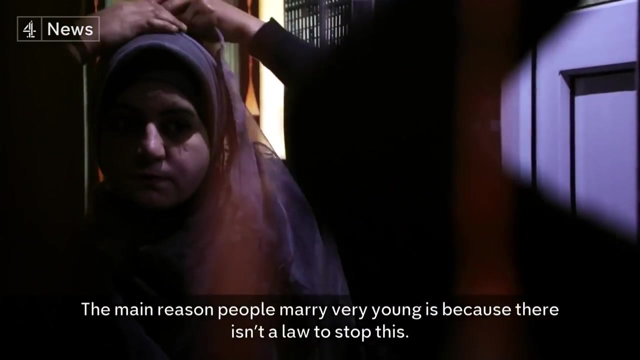 I remember that I wasn't able to look at my eyes. I remember that I wasn't able to look at my eyes. I remember that I wasn't able to look at my eyes And once I would pur that tears and say I'll never look back on it. 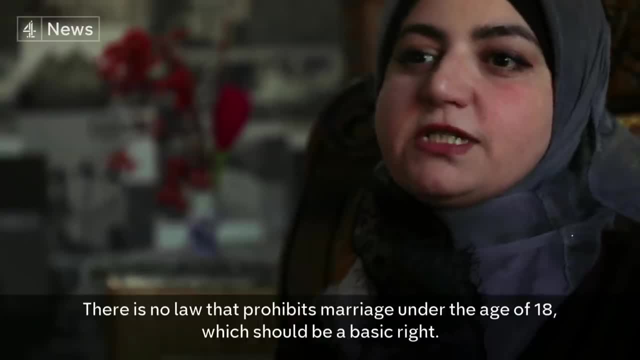 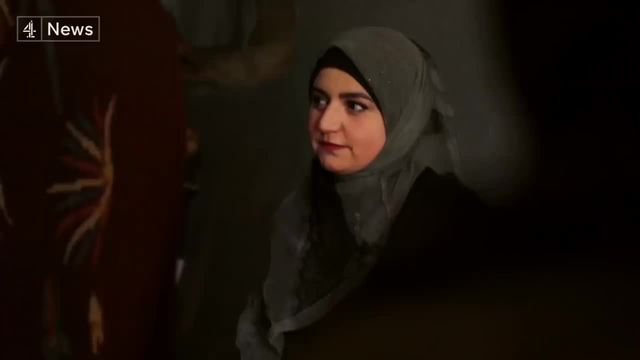 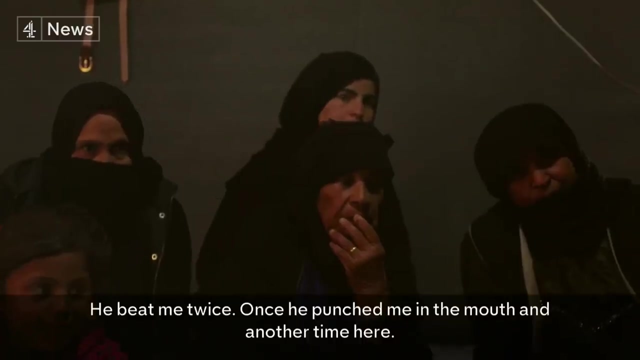 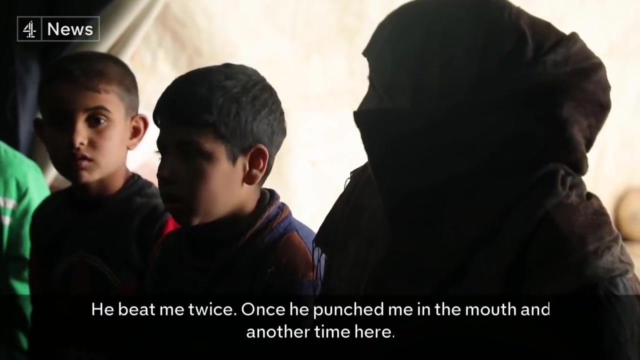 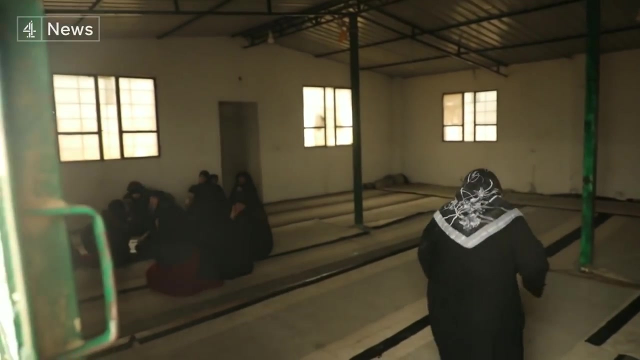 Unfortunately, we don't have a law that prohibits marriage under 18 years of age. This is the main focus and we need to focus on it. Maisa teaches across Idlib. Her lessons are an opportunity for women to share their stories. Maisa's workshops are a stark contrast to the religious lessons the women must attend in camp. 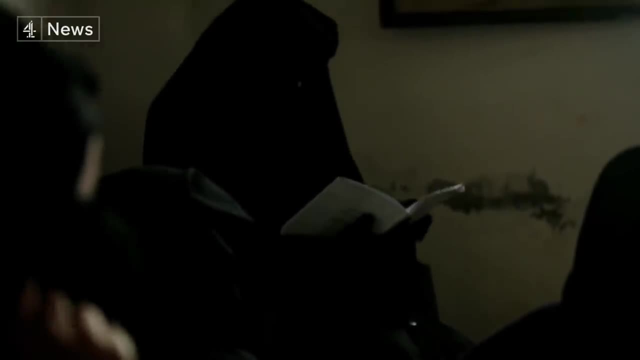 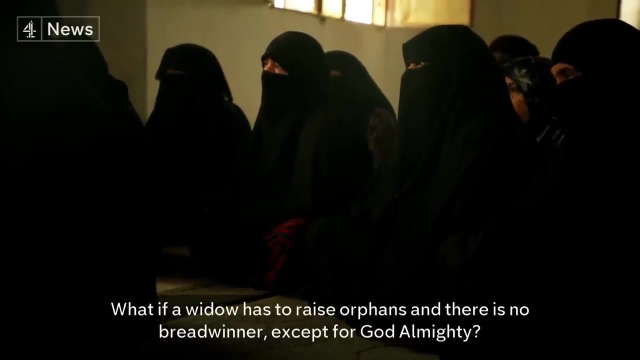 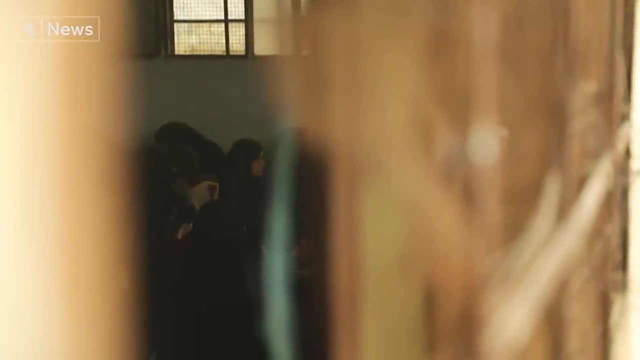 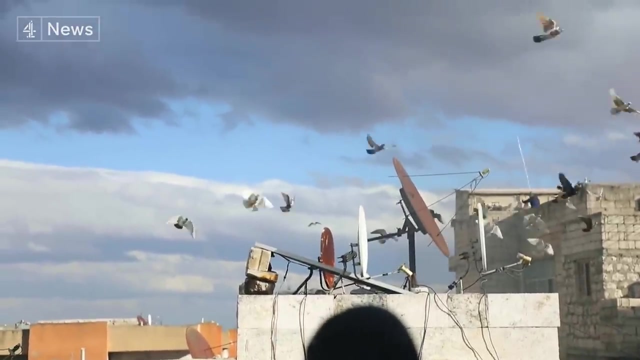 reinforcing and reminding them of their place in the world, always and forever. behind the men. There is no one who can help her except Allah. On an Idlib rooftop, Jamana, a single mother and her children, doesn't even have the safety of the widow's camp.